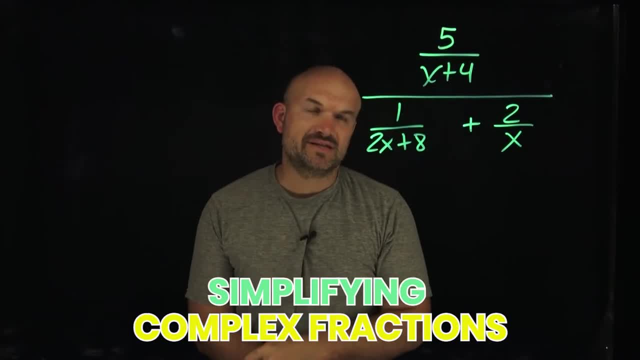 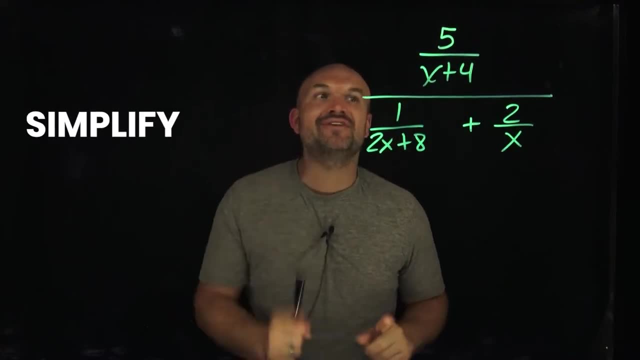 Why don't? the best tip that I can give you for simplifying complex fractions is just to multiply the denominators. But I don't want you to multiply the denominators right here. What I want you to do is simplify first. So what I want you to do when you're first 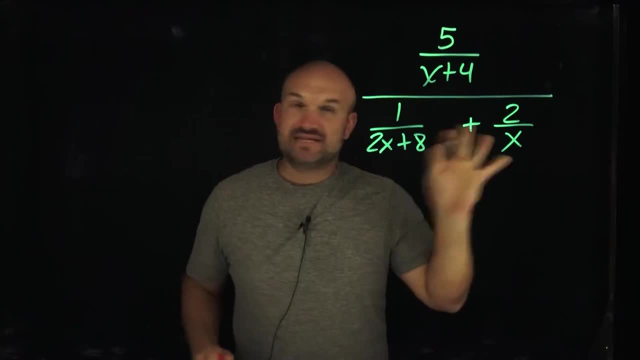 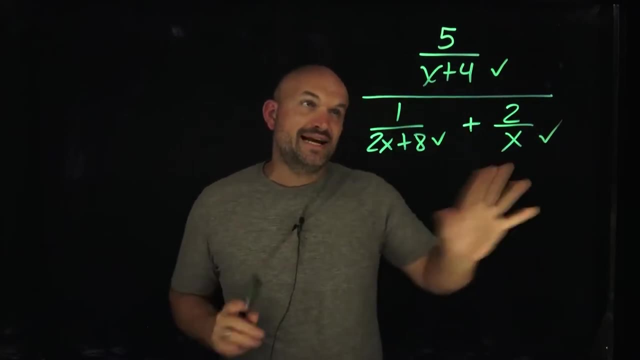 looking at a complex fraction is just kind of like: count all the denominators that you have. right, You have one, two, three, okay, So now what we need to do is say: all right, which of these denominators can I simplify: X plus four can't really do anything Over. 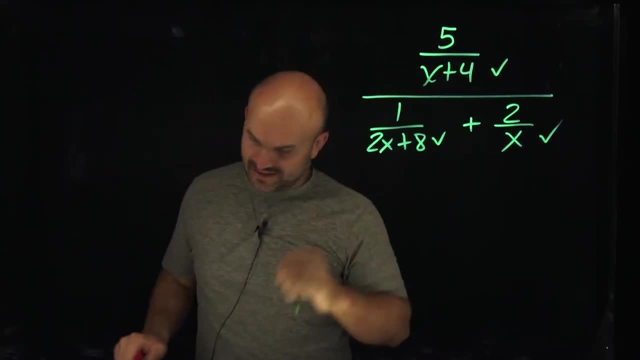 here, though, I know I can factor out a two, So therefore, what I'm going to do is simply: below it, I'm just going to factor out the two, and that's going to be an X plus a four. Okay, Now I'm just going to put a line through there, And then, over here, I have an X. I. 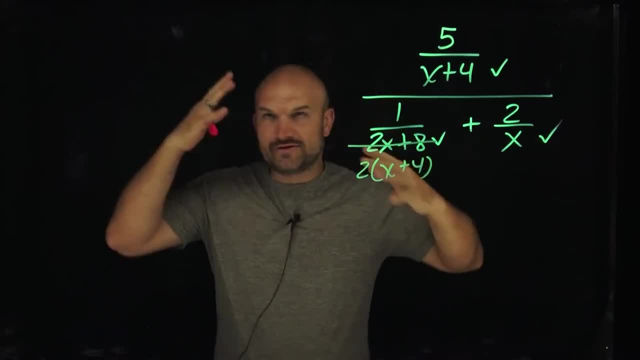 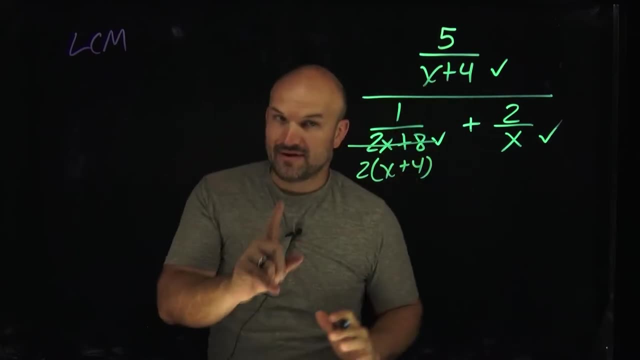 can't do anything from there. All right Now. so this tip: the best thing to do is, instead of trying to remember or trying to think about you know what are the common denominators, is just to multiply them. But here's the caveat, though: You have to first simplify and then 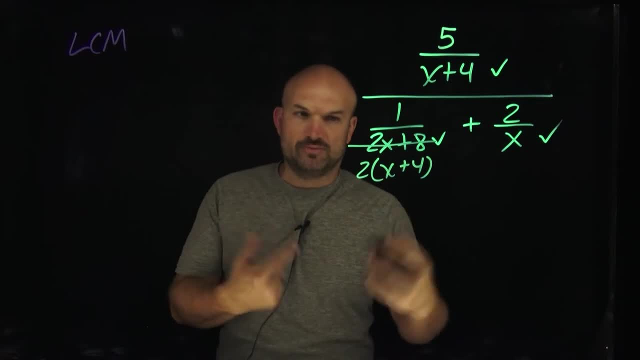 two. you don't need to like re-multiply things Like you don't need to repeat multiples. Right here I have an X plus four and X plus four. I don't need to continue like I don't need to put X plus four squared. 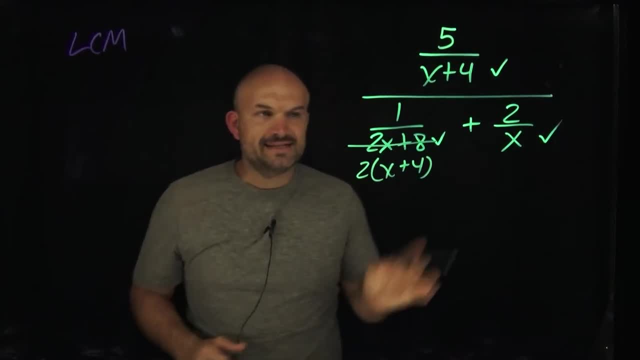 You only need it because you're going to be able to simplify it. And then, two, you don't need to repeat it once, right? Because remember our goal, our idea is, whatever our denominators are, have to evenly divide into our numerators, And what we're going to do is we're going. 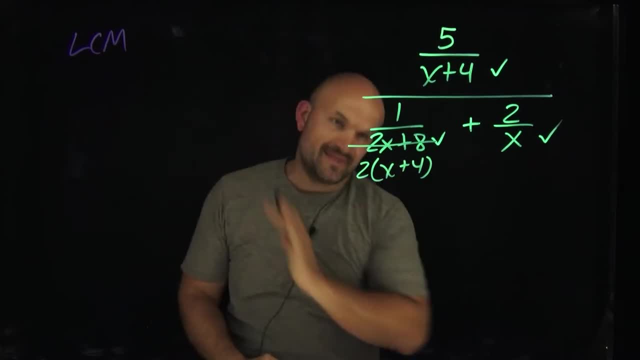 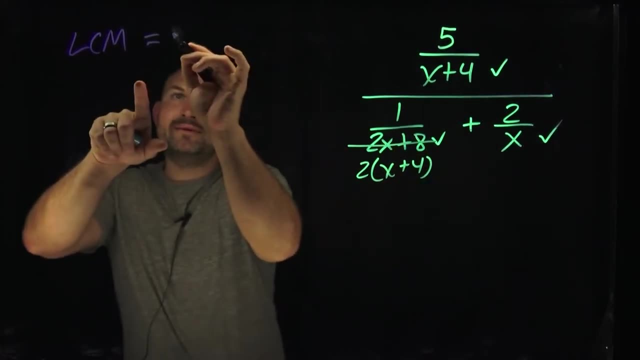 to multiply everything by the least common denominator. That's going to be our numerator. That's how it's going to work. So we have two times X plus four. And then what else could I multiply by An X, right, So I could rewrite my least common multiple as a two. 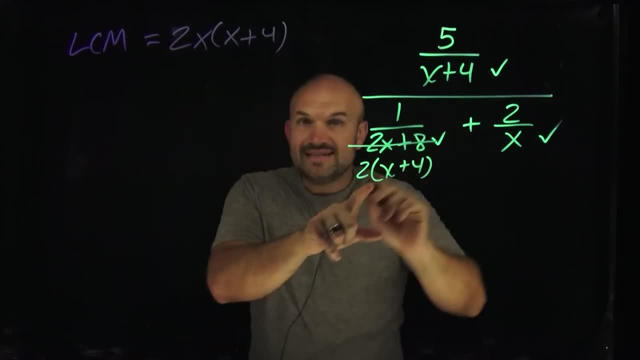 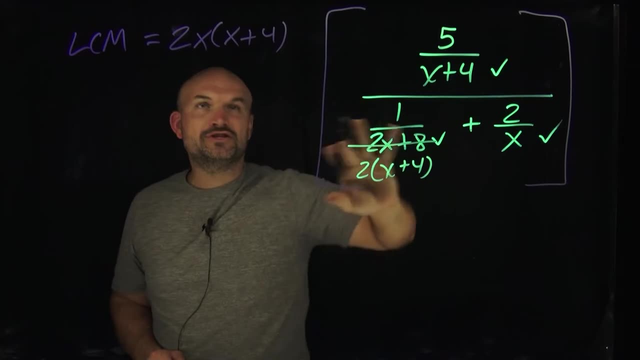 X times an X plus four. All right Again, I don't need to apply this twice, So what I'm going to do is I'm just going to put brackets here. Now, this is a pretty big problem, and I'm not going to want to rewrite every single term. times this two X plus four, but I just 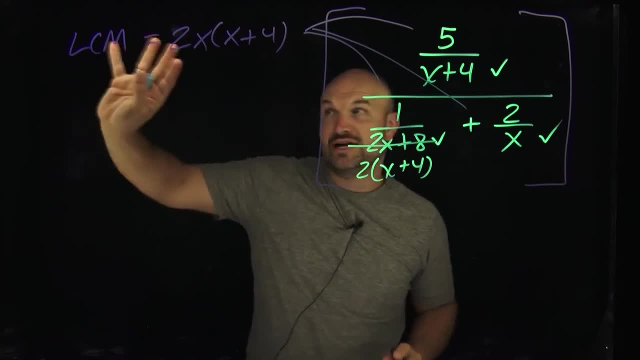 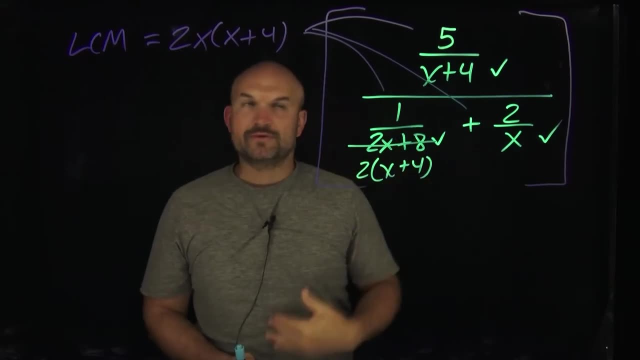 want you to understand. you're going to multiply this the two X times X plus four, your LCM times, everything over here. So I'm going to do a little bit of mental math gymnastics here And, as we're applying it, kind of talk my way through so you can follow along. So 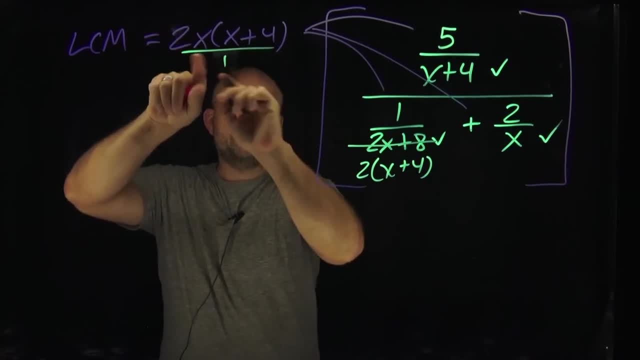 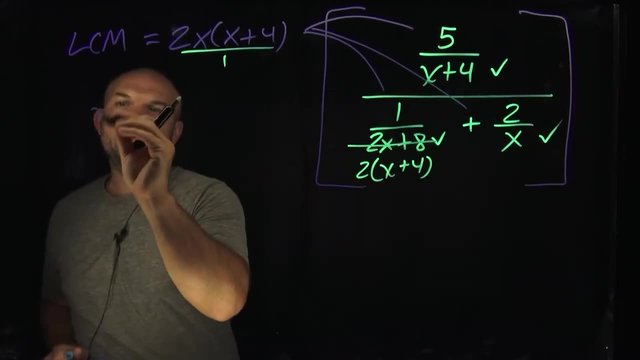 when I multiply a two- X, remember this is technically over one, right? So I multiply two X times X plus four times the five over the X plus four. the X plus fours are going to divide out And that's going to leave me with a two X times a five. 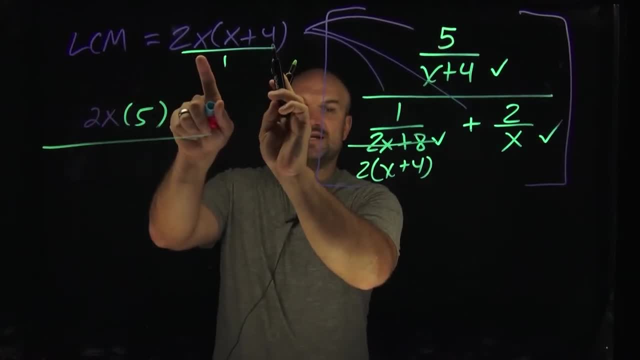 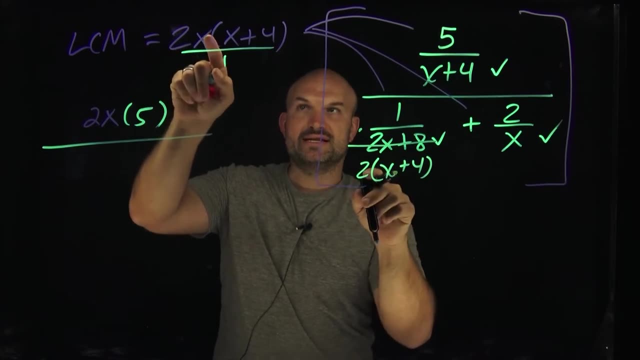 All right, Then let's go to the next one. here I'm going to multiply two X times X plus four times a one over two times X plus four. So the twos are going to divide out, right, Because this is the numerator, this isn't the denominator. So the twos will divide out. 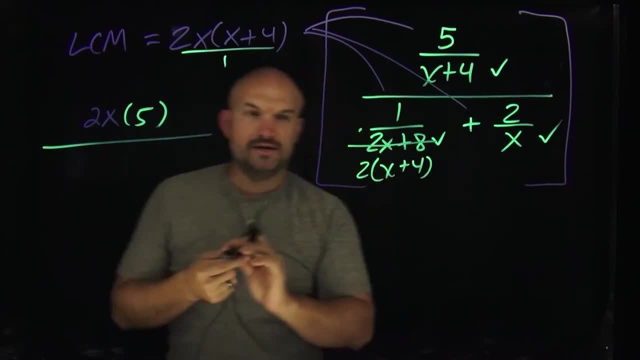 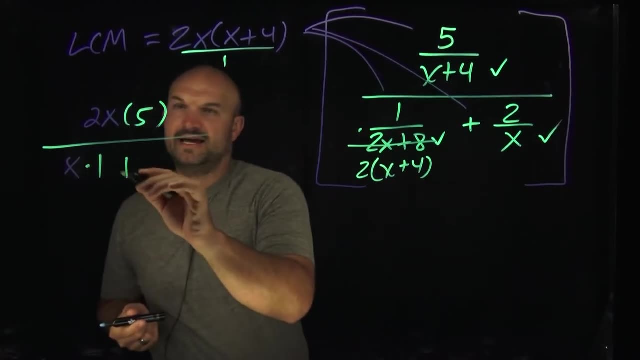 and my X plus fours will divide out. That's just going to leave me with an X times a one. So therefore I'll just write it like this: an X times one, And then over here we're going to have a two X times X plus four times a two over X. Well, here the Xs are going. 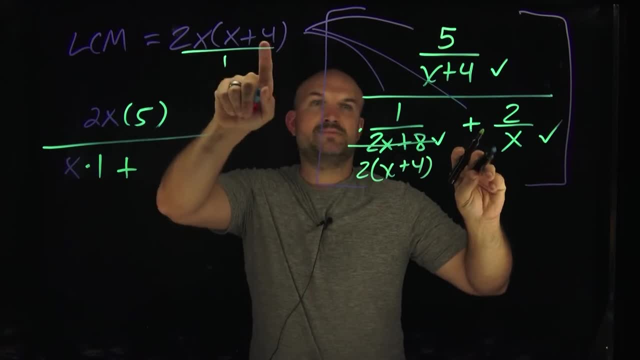 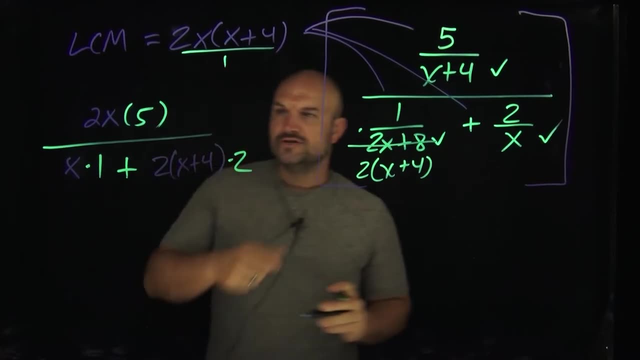 to divide out and that's just going to leave me with a two X times X plus four times a two over X. So that'll be a two times an X plus four, and then times two. Okay, So now you can notice here. what happens, guys, is remember all these denominators that I had right This one. 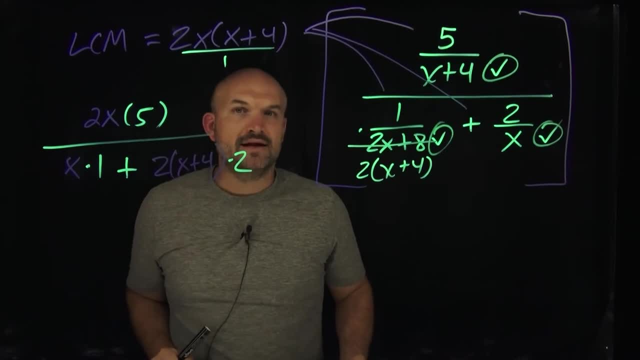 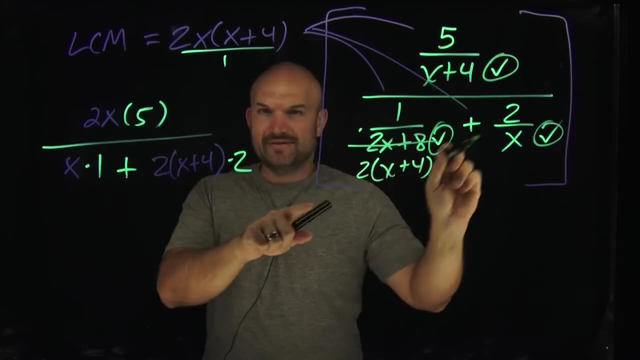 this one, this one. If you multiply your least common multiple, correct, then you will have gotten rid of each and every one of your denominators right. And notice, I got rid of them. That got rid of, got rid of, got rid of. And the reason why you didn't really like get rid. 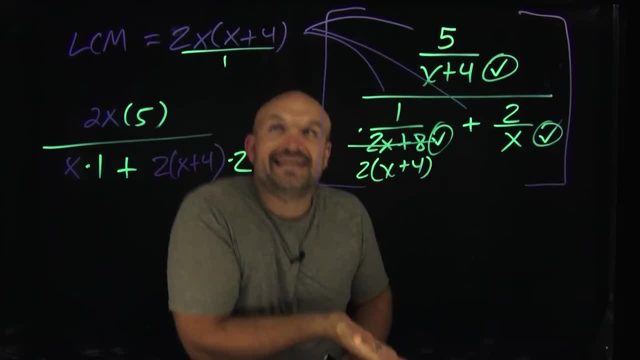 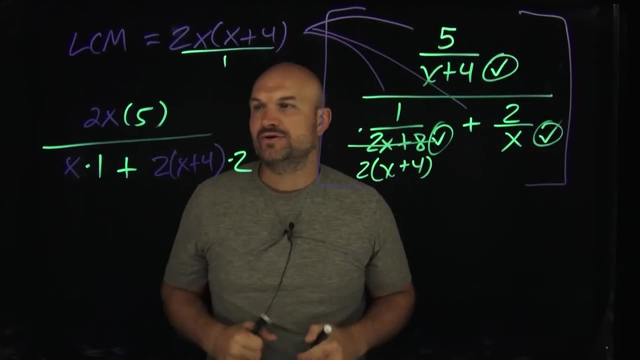 of them all. what happened was your least common, your denominators divided out, They divided evenly into this least common denominator that you multiplied. And as long as you multiply everything by the least common multiple, you're not changing the value of your complex fraction. Now we need to go into simplify things. So I have a two X times five. 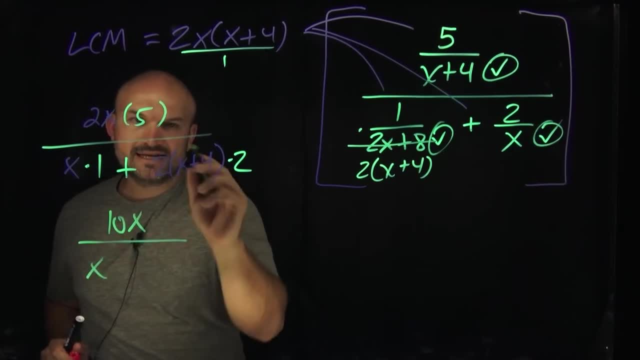 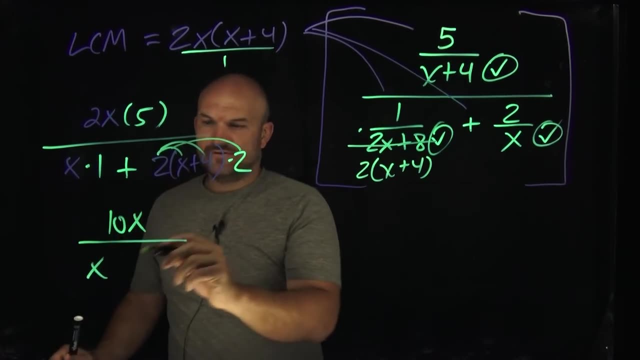 which is going to be a 10 X. That's going to be all over a X I can distribute here. So that's going to be actually you know what. Let's multiply the two times two is a four. So therefore that's going to be plus a four X and that'd be plus 16.. Cool, And now I can. 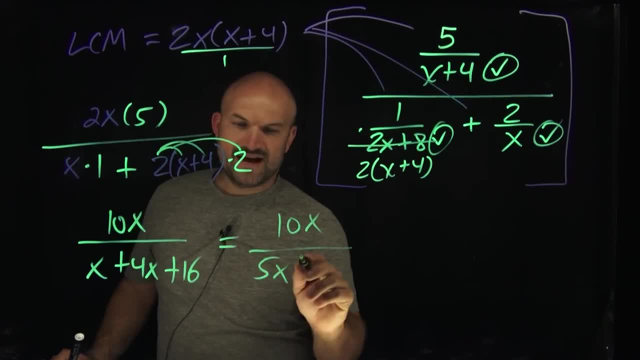 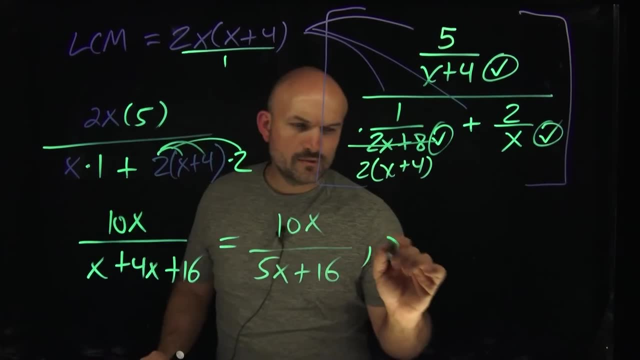 rewrite this as a 10 X all over. Let's see what is that going to be: A five X plus a 16.. And now let's go and look at our values that are going to be restricted. So when you're dealing with the complex fraction, 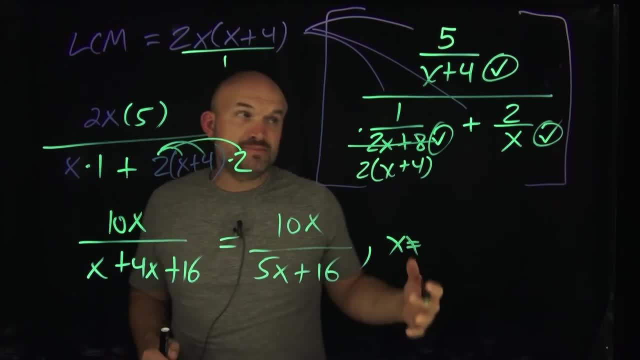 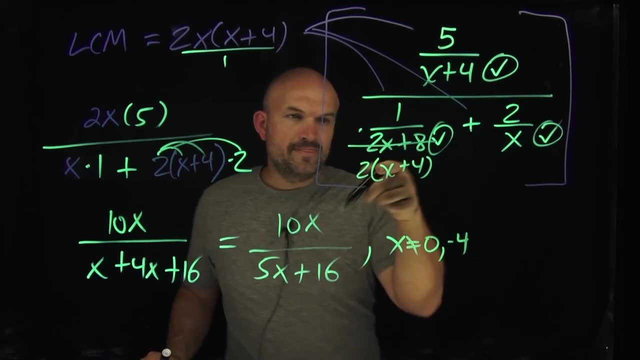 what I always like to say is: like: all right, what are the values that X cannot equal? All right, Well, those are going to be the values that are going to make your denominator equal to zero. So you could say: X cannot equal zero, right, X cannot equal a negative four. This: 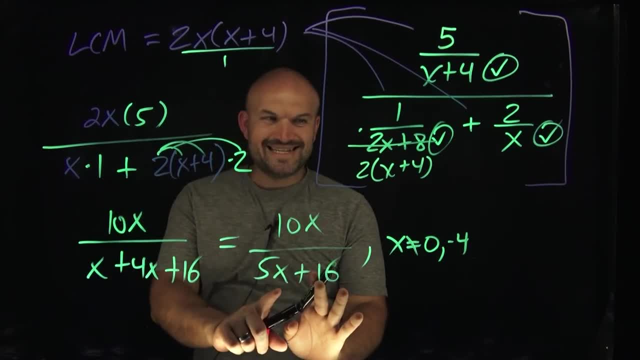 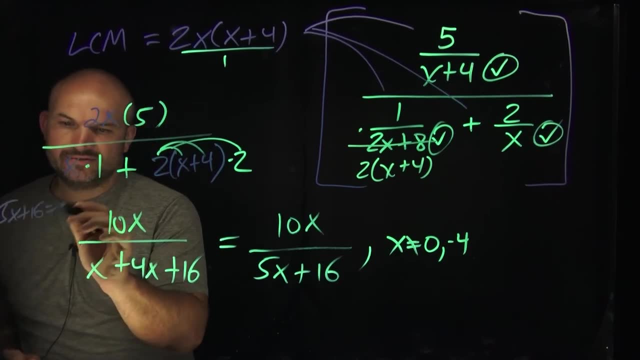 would be the same thing. And then also here: if you were to set a five X plus 16 equal to zero, what would that be? Well, again, let's just kind of do the work over here. You know, if I had a five X plus 16 equals zero,